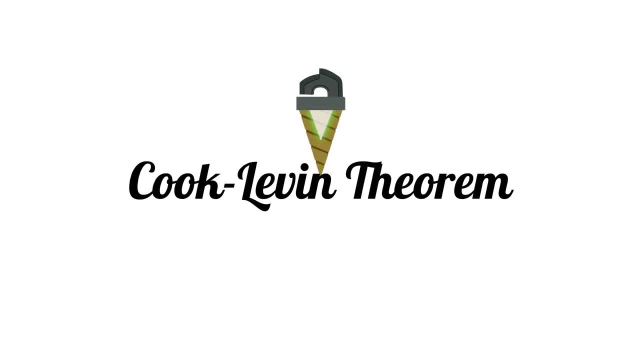 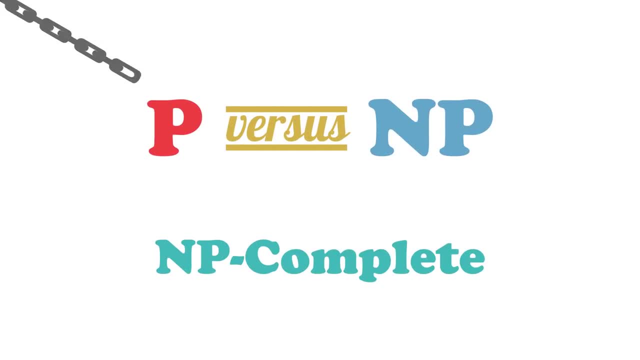 using a problem called SAT. Before we dig in to how they did this, let's look at the implications of this result. P vs np is bound to these np-complete problems. If p equals np, then np-complete problems are in p, and if np-complete problems are in p, then p equals np. 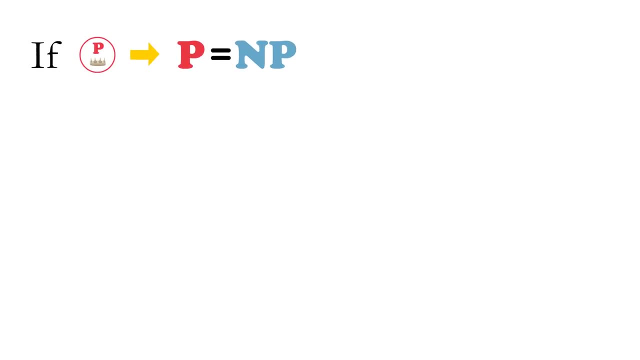 The reason is pretty simple. By definition, np-complete problems can be used to solve any problem in np. Thus, if an np-complete problem is easy, all of np is easy. Conversely, if np is easy, then np-complete problems must be easy, since they are part of np. This relationship 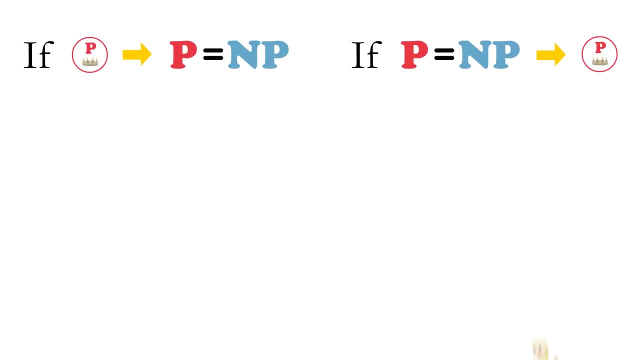 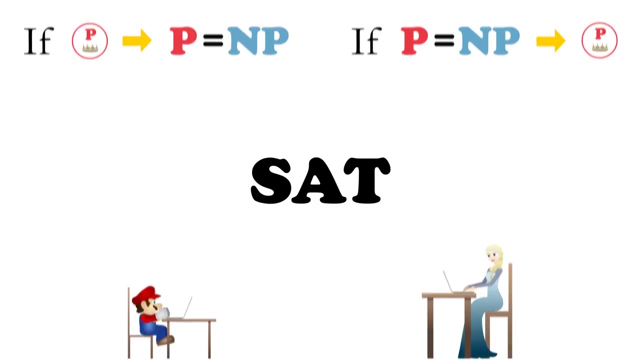 is important because to solve p vs np we only need to focus on a single np-complete problem, as opposed to the giant set as a whole. Going back to the Cook-Levin theorem, we're going to look at a version of SAT called circuit. 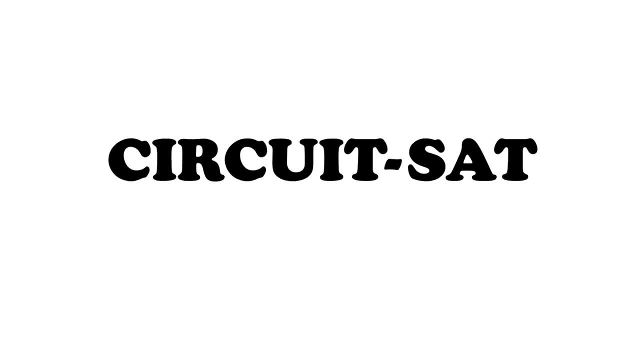 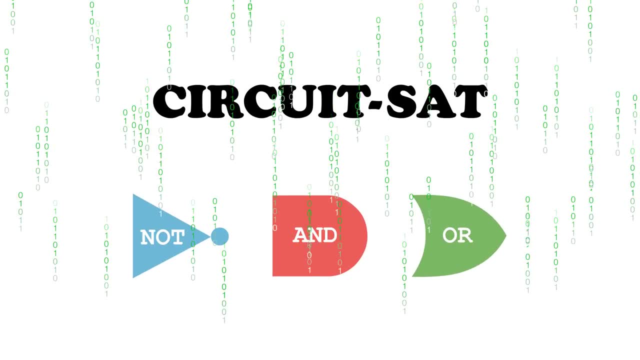 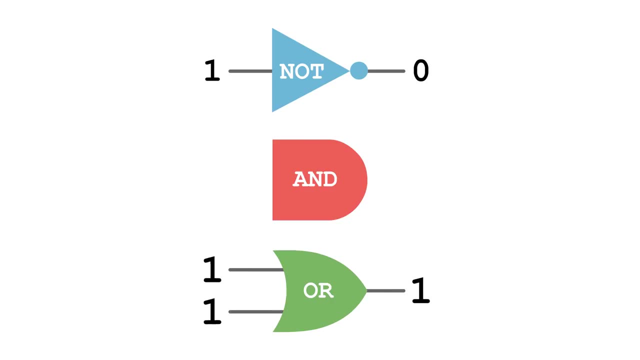 SAT or the circuit satisfiability problem. In this problem we're given three types of circuits: the NOT gate, the OR gate and the AND gate. Inputs can be either 0 or 1.. The NOT gate flips 0s to 1s and 1s to 0s. The OR gate outputs a 1 if any input is 1,. 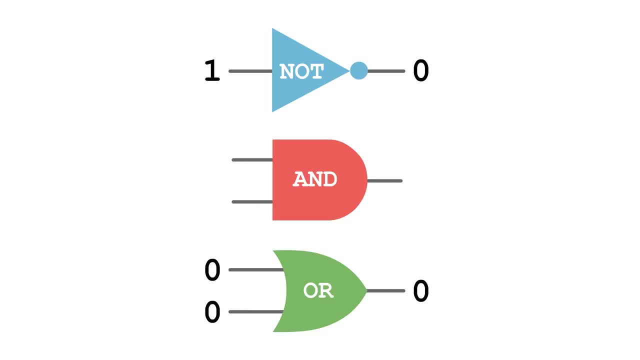 and outputs 0 if all the inputs are 0.. The AND gate outputs a 1 if all the inputs are 1, and 0 if any of the inputs are 0. We can stick the circuits together like LEGO pieces to create larger, complex circuits. The circuit SAT problem is to tell for a given circuit. 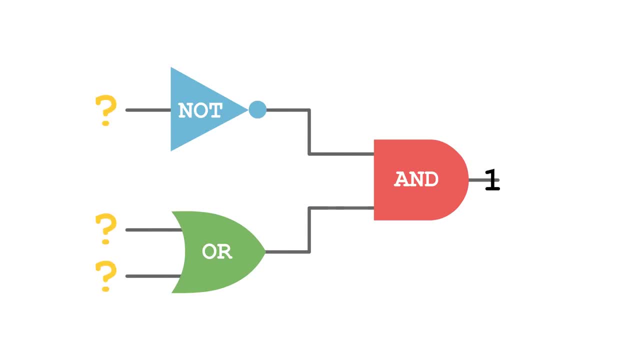 whether or not there is some input that will eventually output a 1.. The brute force solution for solving this problem is to just try every possible input. Since each input can be either 0 or a 1, this gives us 2 to the n possibilities to try meaning. 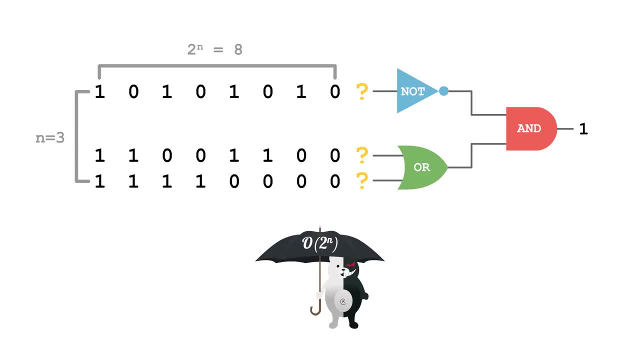 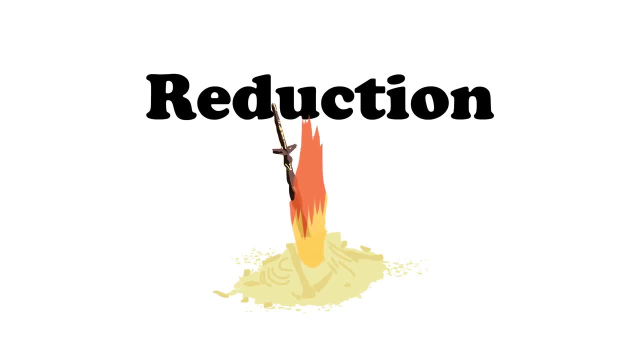 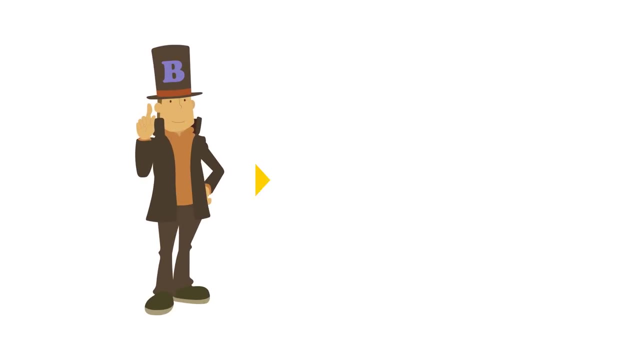 our brute force. solution takes exponential time. This problem seems challenging, and we're going to prove that indeed it is, using a technique called reduction. We say that problem A reduces to problem B. if we can use a solution for problem B to solve problem A, If we can show this, then solving B kills. 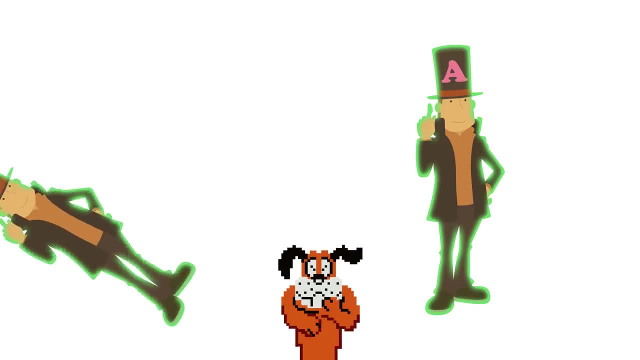 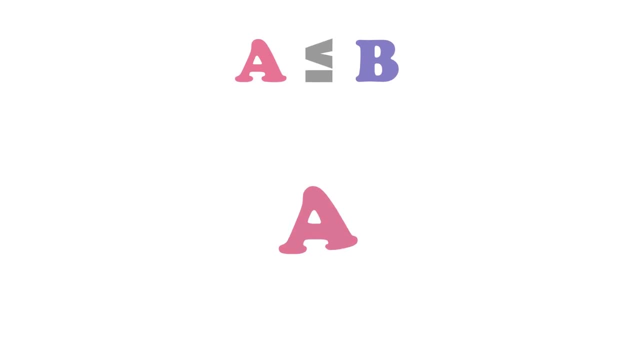 with one stone, We've found a solution for both B and A, meaning that A is no harder than B. Typically, we do this by providing a quick conversion from problem A to problem B. Our A-solver would then look something like this: Take an instance of problem A. 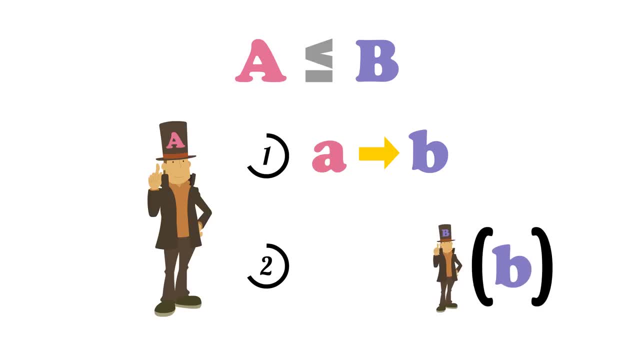 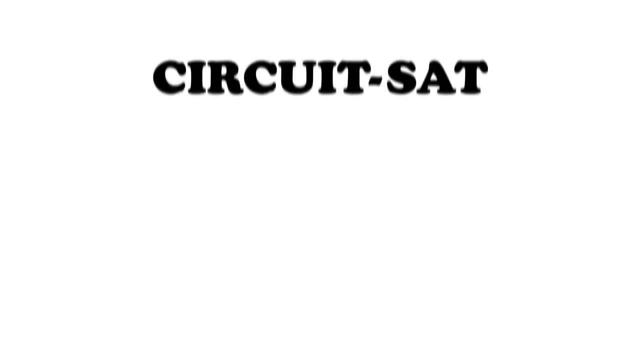 convert it to problem B, use the B-solver to get a solution and finally use that solution for problem A. Remembering that circuit SAT is the hardest problem in NP is a bit tricky because we aren't converting from one problem to another. We need to somehow convert all NP problems into. 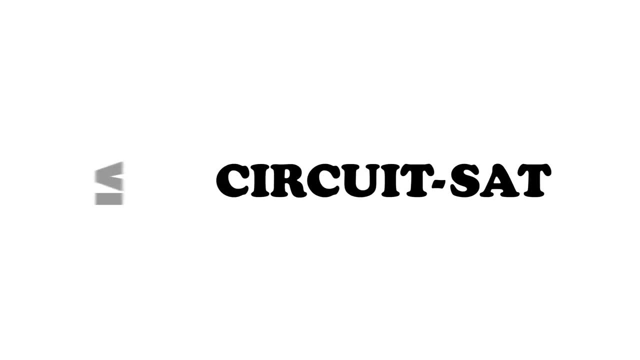 an instance of circuit SAT. If we can somehow do that, we could then crown circuit SAT as the hardest problem. Remember from our NP video that one of our definitions of NP is that there exists a verifier that runs in polynomial time. A verifier is: 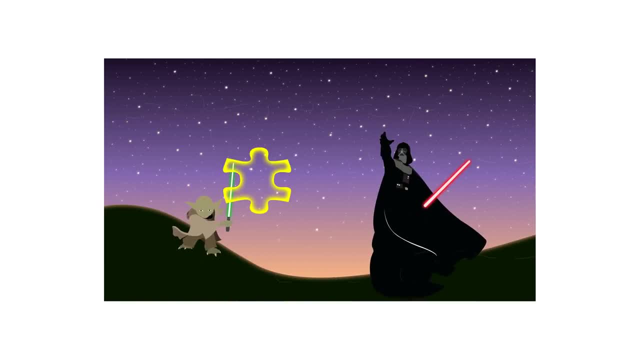 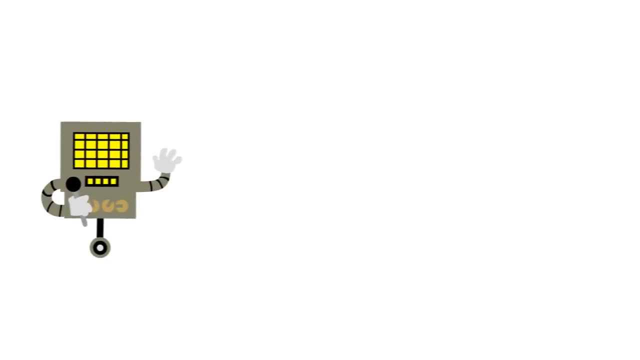 a special program that takes a proposed solution and can quickly confirm if that solution is correct. Our plan of attack is to take an arbitrary verifier program and encode it as a circuit. This would allow us to convert any NP problem into a circuit by using its. 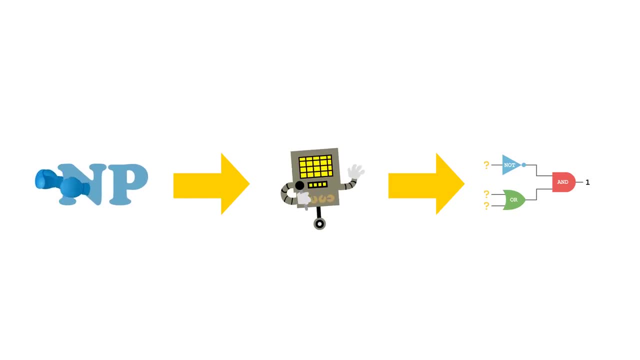 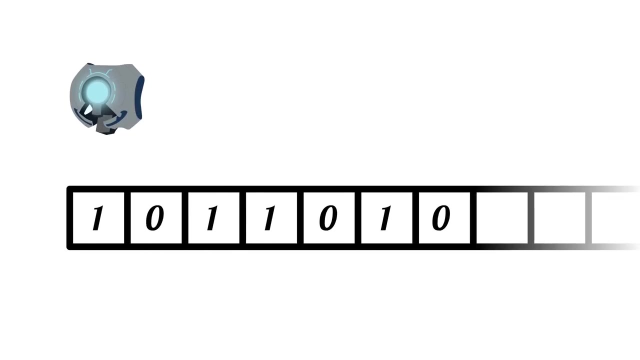 verifier program as a proxy. However, we need some type of model to describe the verifier program. For this video, we're going to use the Turing machine. A Turing machine is a very simple model for computation. The machine is an infinitely long tape broken up into cells which either contain a one, a zero or nothing. The tape 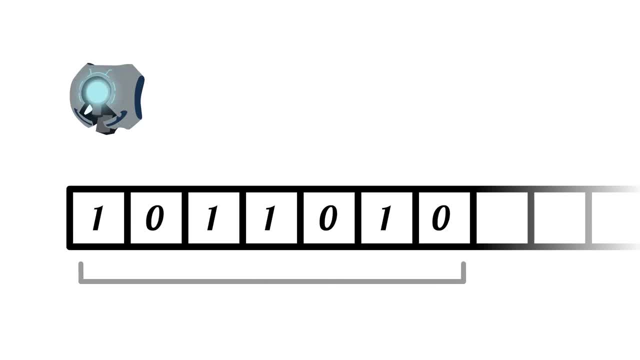 initially begins with a series of 1s and 0s, which represents the input for the program. The machine also has a head which is over one of the cells. Every step of time the head will read what is in the cell it is over. The machine can then decide what to write in. 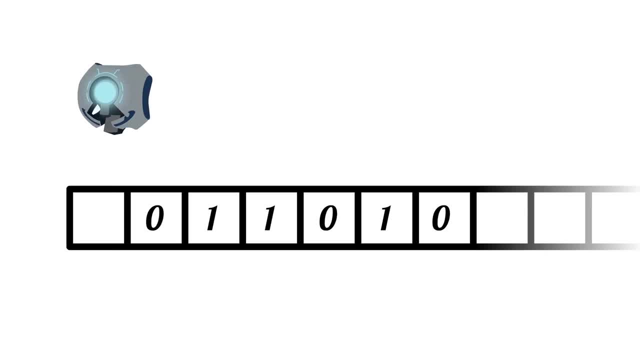 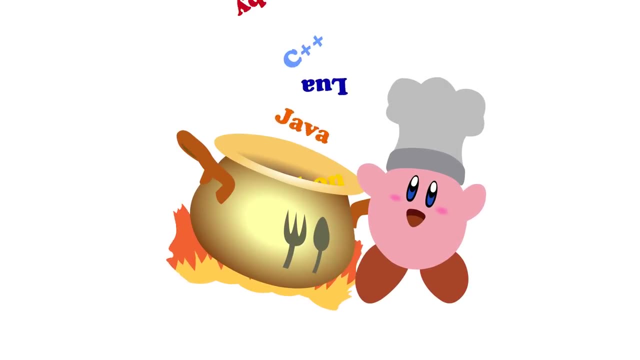 that cell either 1,, 0, or nothing, and then move over one space to the left or the right, Based on its execution, the machine will finally decide whether to accept or reject the input. This doesn't sound like a lot, but all modern programming languages boil down to a version. 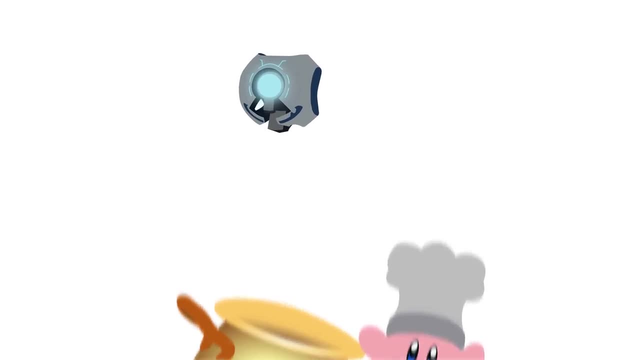 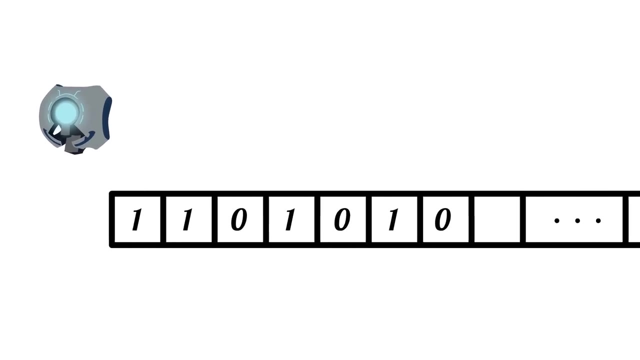 of the Turing machine. Now we want to convert our verifier Turing machine into a circuit. The initial Turing machine starts with a tape and its input. Let's use this one as an example. Normally, a Turing machine can go on for an infinite length, but the verifier for an NP. 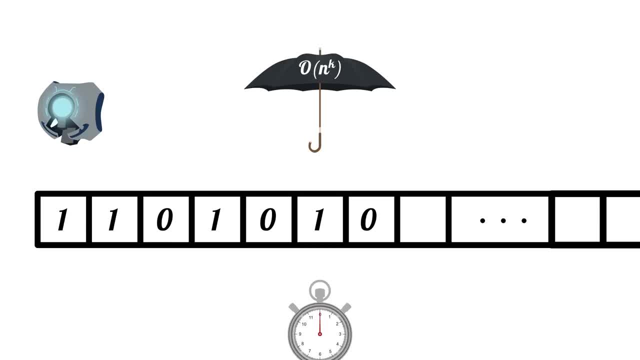 problem must run in polynomial time, And since a Turing machine can move at most one cell per timestep, we only need at most end-of-the-case cells. For illustration, let's say that after one timestep the machine will turn the first cell into a zero. 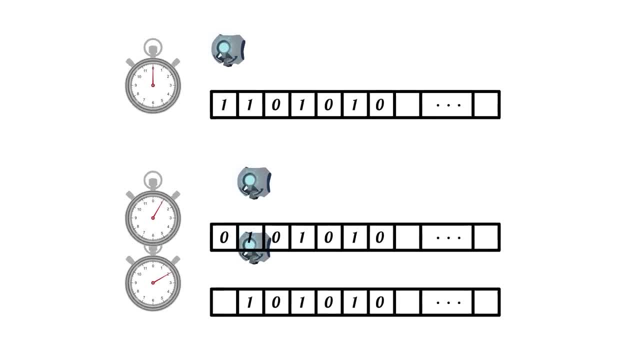 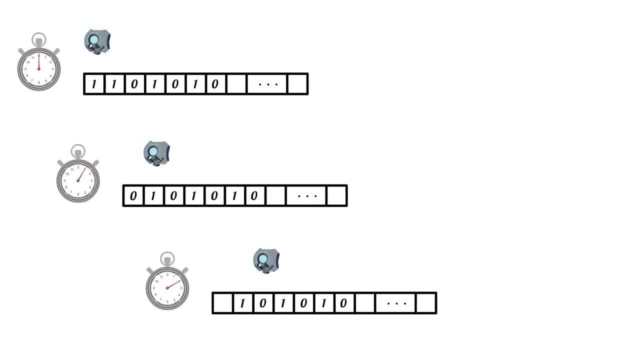 And move one cell to the right After the next timestep. let's say that the machine keeps the second cell as a one and moves to the right again. What we want to do is convert each timestep into a row of circuits. The initial tape acts as an input into our first row. 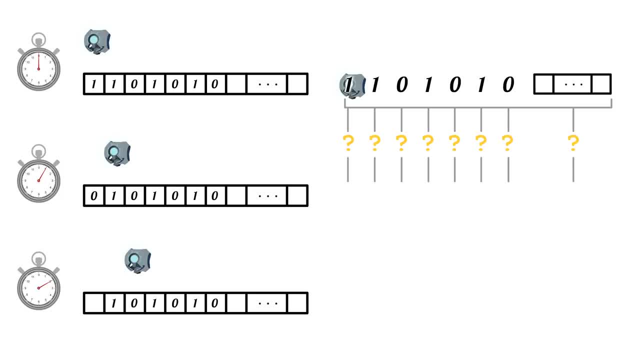 The row of circuits, then churns through the ones and zeros and eventually spits out a sequence of outputs that matches what the tape looks like after the first timestep. We want each new row of outputs from the circuits to correspond exactly with what the Turing machine tape would look like after that many steps. 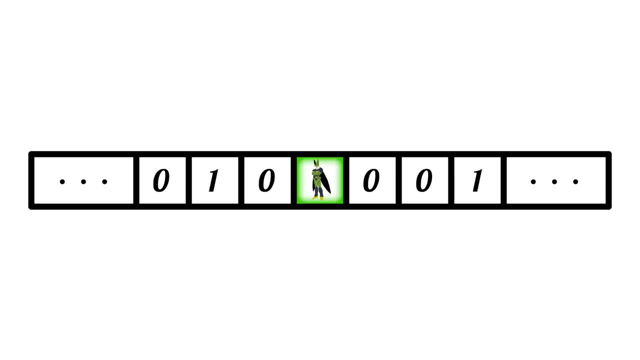 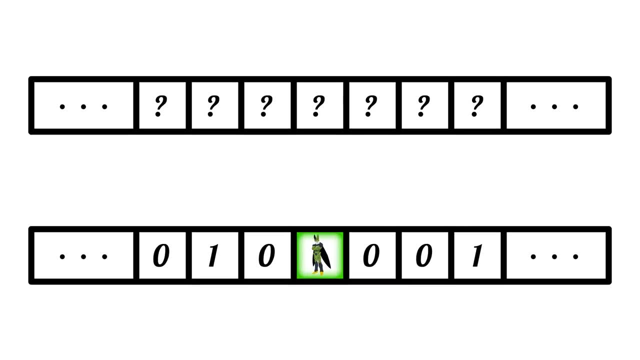 Looking at an individual row for cell I, how do we know what the cell should look like? It's important to note that cell I at a specific timestep is only based on three cells From the previous timestep. it can be influenced by the cell at I or the cells immediately before. 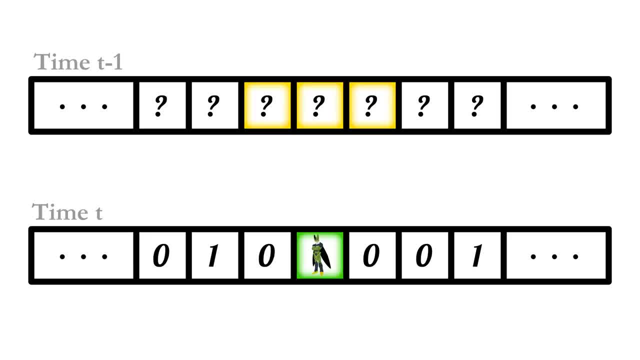 or after it. The cells before and after matter because the head of the Turing machine could potentially move into cell I from either of these two cells. If the head was on cell I, then the element might also be flipped to one or zero. Otherwise cell I is guaranteed to stay the same. 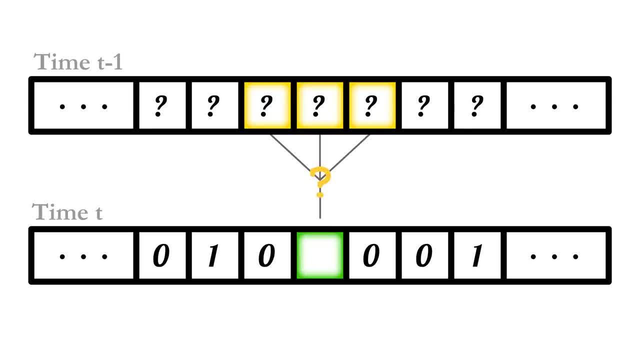 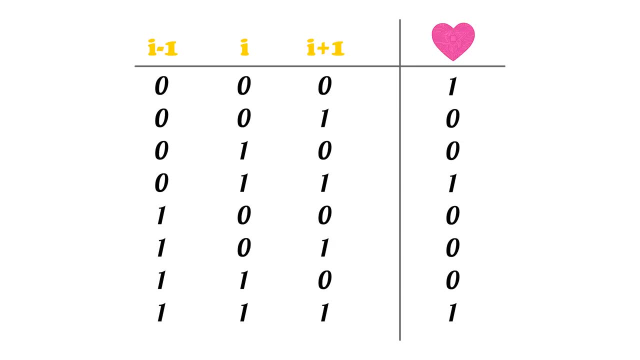 So we want to build a circuit taking these three cells as input, which we'll visualize with this heart circuit. I won't go into the specific details of how the heart circuit works, but you can imagine one that hardcodes all of the possibilities given the three inputs. 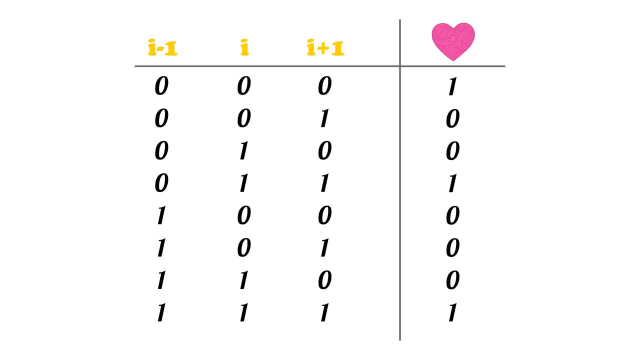 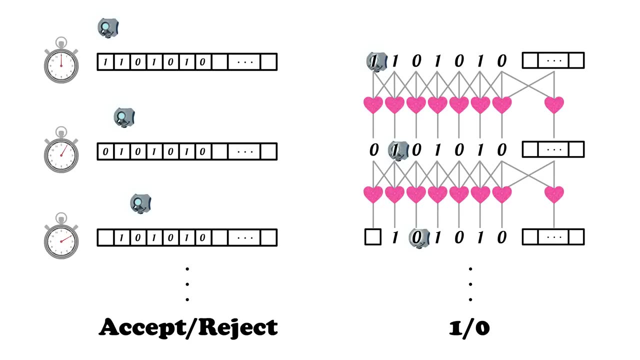 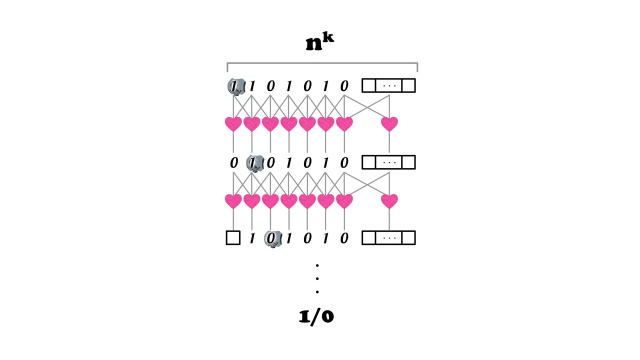 It would use a bunch of circuits, but it's a fixed size. We can now fill in the overall circuit with a bunch of heart circuits to convert from row to row. How big is our overall circuit? Well, since the tape has N to the K cells, 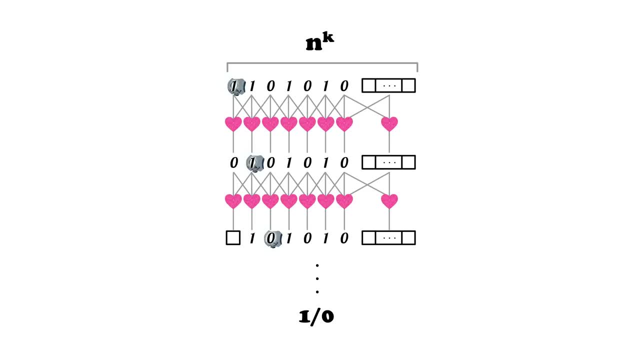 Each row of our big Turing machine tape has N to the K cells. Each big circuit will have N to the K of these heart circuits. We also have N to the K rows of circuits, since each row represents each time step for the polynomial time algorithm. 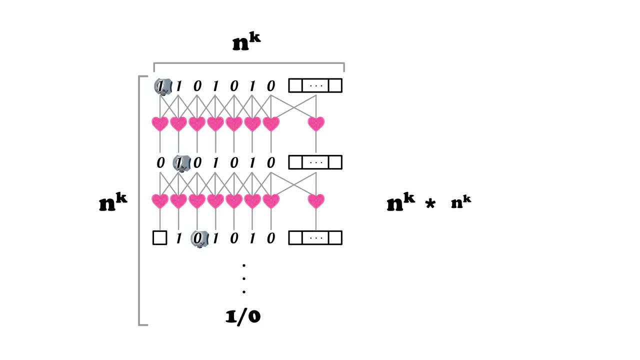 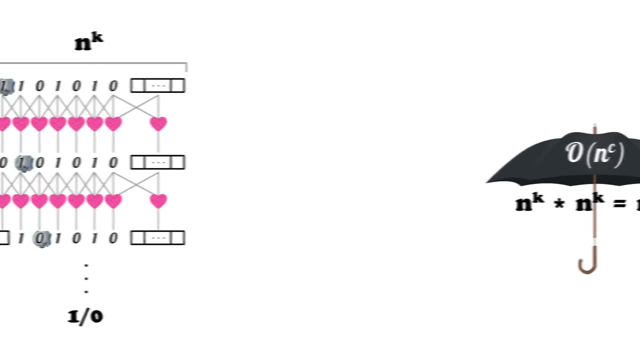 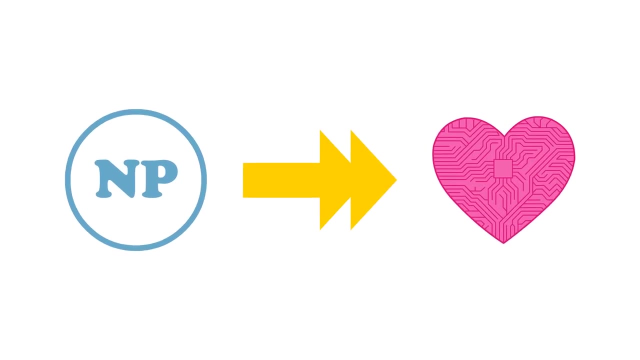 This gives us a total size on the order of N to the K times N to the K or N to the 2K, which is still polynomial. This gives us a polytime conversion from an arbitrary NP problem to a circuit. This circuit is a fairly direct emulation of how the verifier algorithm works. 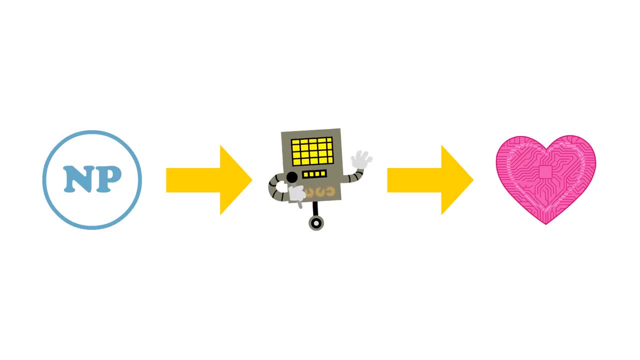 To easily solve a problem in NP, we need to be able to figure out if there's an easily verifiable proof for that problem, For the problem of whether a Mario level is beatable. we want to know if there's a sequence of inputs that will eventually get Mario to the flag stand at the end of the level. 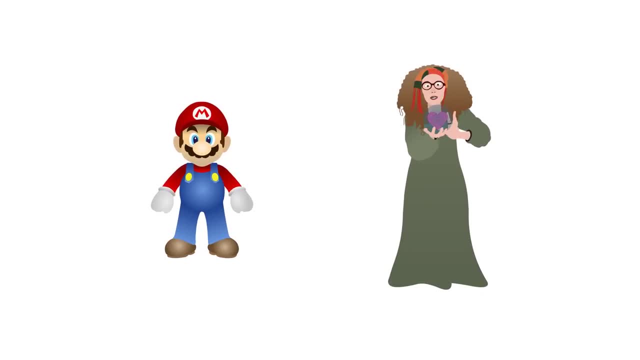 If we had a circuit set Oracle, we could easily solve the Mario question. We take the term N to the K and we can easily solve the Mario question. We take the term N to the K and we can easily solve the Mario question. 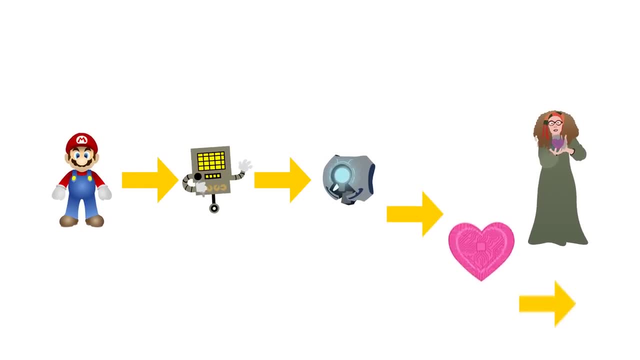 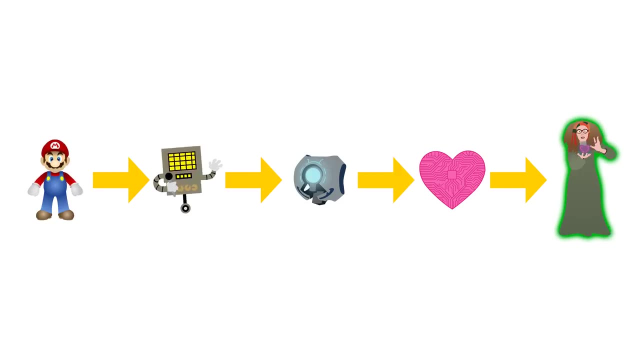 nauc Gibran acted as a scrolling machine that verifies the Mario inputs and turns it into a circuit, as outlined in this proof sketch: The circuit set. Oracle will then tell us whether or not the circuit is satisfy-able, which maps directly to whether or not there is some sequence of button inputs that will beat the. 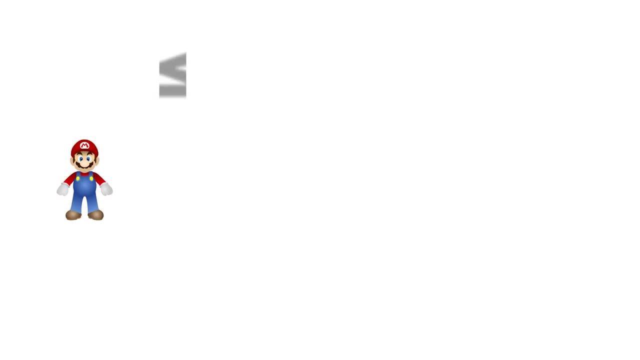 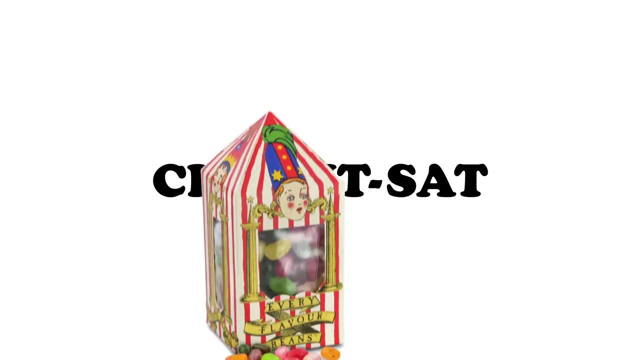 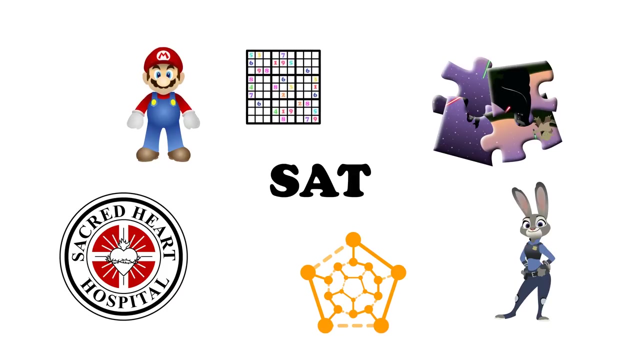 Mario level. This tells us that CircuitSat is at least as hard as the Mario problem. The first problem to have been proved to be NP-complete was a flavor of CircuitSat just called Sat. We now know of hundreds of NP-complete problems, While the first one had to go through this convoluted process of reducing all problems. 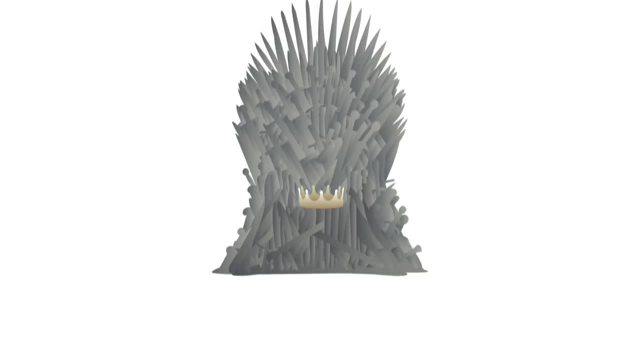 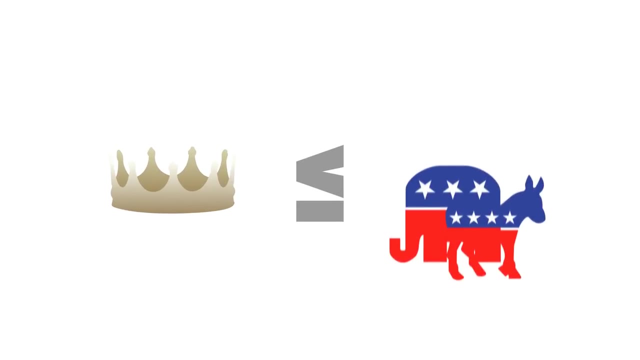 to NP into SAT. it's a lot easier to prove a problem is NP-complete. now We just need to take any existing NP-complete problem and reduce it to our candidate problem. This would make our candidate at least as hard as a problem we already know is the hardest.